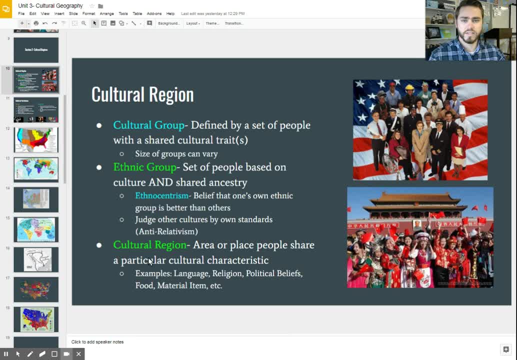 another good example of that. However, it's not necessarily the case in all countries. You see, the United States, for example, were a mix of many different ethnic groups, and so, while it can be an entire country, population is not always so careful on that distinction. there You have to share a common ancestry, a history. 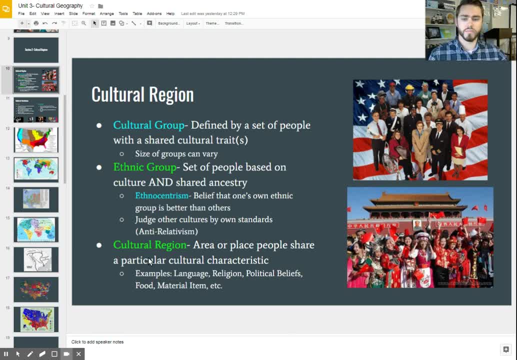 as well as a culture. Okay, The other term I want to talk about when we're talking about ethnic groups is ancestry ethnocentrism. okay, you may have heard this term before. basically, it just means that you believe that your ethnic group is better than others. you believe that you know others are inferior. 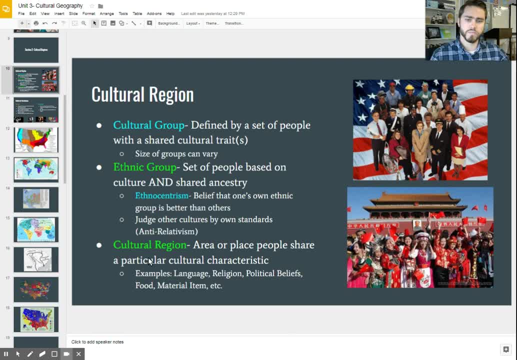 to your particular culture and shared ancestry and somehow, some way, you are better than others. and while this can be very mild, in an example it could be, you know, having pride in your country and just believing that you are great. you know, that's a very mild form of ethnocentrism. it's. 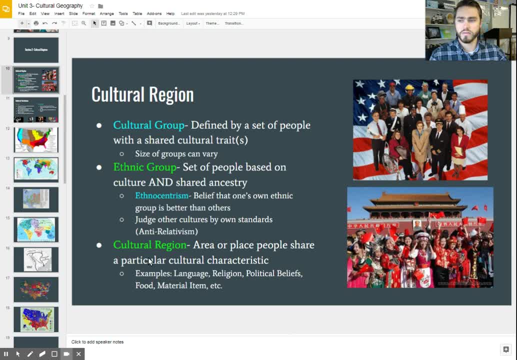 actually, you know, practiced in many countries. you know it's often confused with patriotism and it can also be very, very extreme in the case of, you know, many places around the world you see extreme ethnocentrism leading to persecution of others, the elimination of certain ethnic groups. 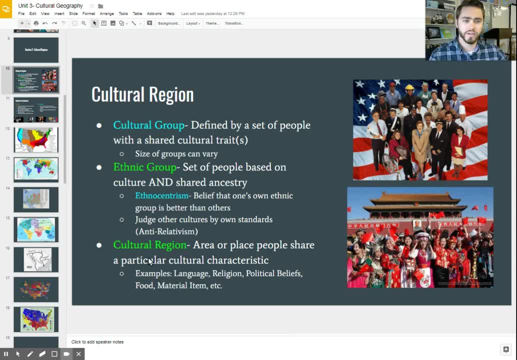 most famously, probably, you might believe, is the holocaust where nazis, you know, targeted certain ethnic groups, particularly jews, gypsies, you know, and other people such as poles and others, and they persecuted them and exterminated large groups of ethnic groups simply for that shared common ancestry, that cultural bias that they had. they believed that. 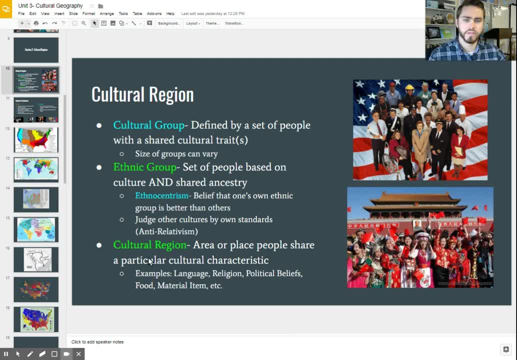 their, you know, ethnic group was better than others, and that others should be taken out of the world for their identity and their identity as a human being. so you know, it can be very mild, it can also be very extreme, and the common trait that you see here is this lack of relativism. 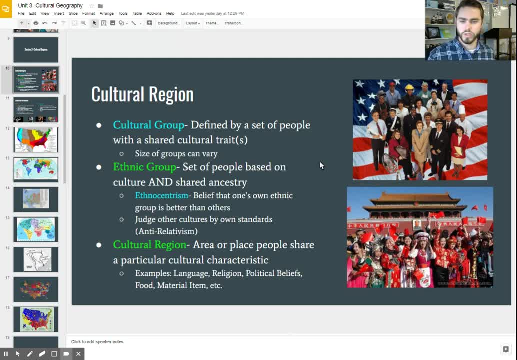 which is a term we talked about earlier in the unit. but remember, what seems normal to us is not normal to other people, and vice versa. you know what other people's normal laws normal is often seems strange to us, and so we have to judge them not based on what we understand is normal, but what 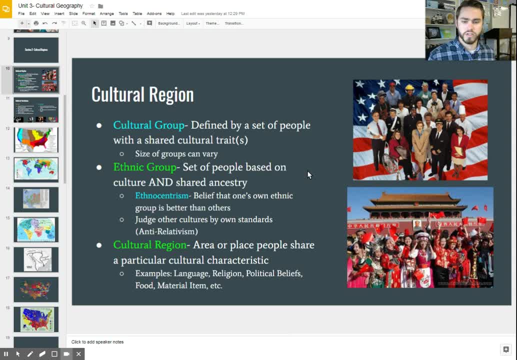 are different. we can't compare them without putting ourselves in their shoes, And if you don't do that, oftentimes what it leads to is ethnocentrism- this belief that your culture is better than others, And that's a dangerous and slippery slope that you can fall into. 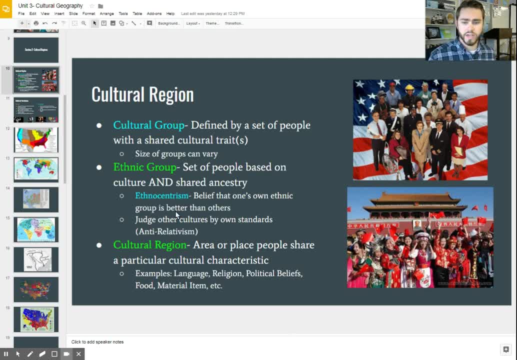 So, like I said, it could be very mild. like you know, just patriotism is a form of ethnocentrism And the other side of the spectrum is extermination of other ethnic groups, And so you have to have this sense of relativism when you're talking about different ethnic groups. 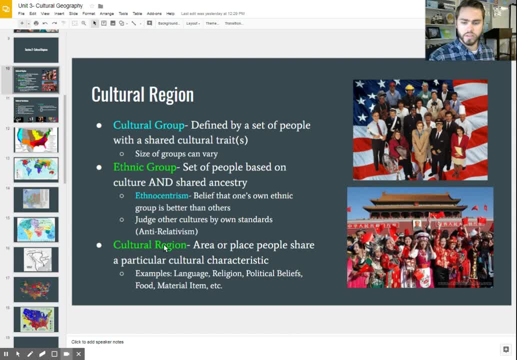 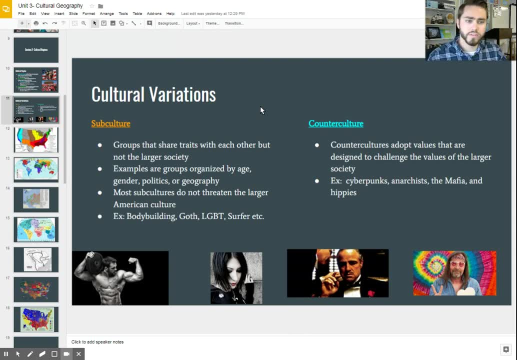 All right, And again we're going to take a look at more in this unit: the different cultural regions. Let's try to map those things out. Before we get to that, let's talk real quick about some other parts of culture that we're going to take a look at today, And this will 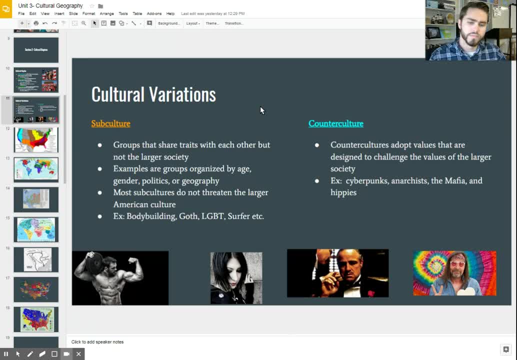 help us to understand ethnic groups and cultural groups a little bit better. There are two subtypes that we'll talk about: a variation of culture Within the larger set of culture. we call these subcultures and countercultures. Subcultures are within an entire population such as America, You have groups that are 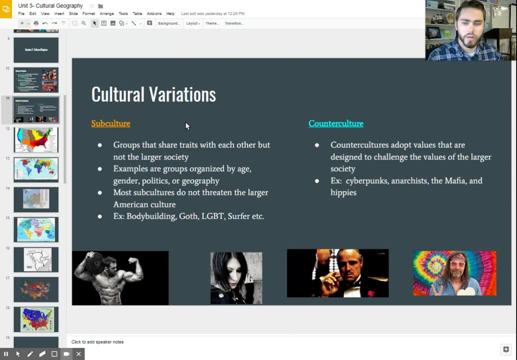 slightly different. They vary a little bit. They have many of the same traits as the rest of the country, but in some ways they are very different. This oftentimes is denoted by their interest or something that you know they share that are different than other people. 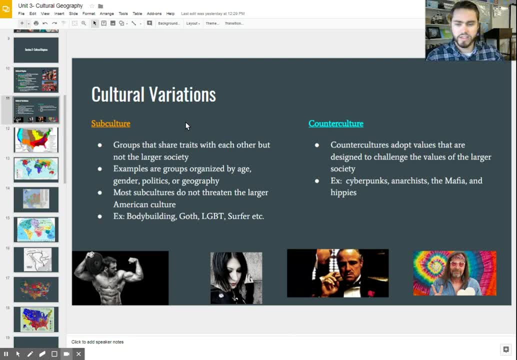 in that country. You know it could be a mix of different ages and genders, but typically they share some particular cultural trait in common that most other people in that country do not. For example, if you're talking about an American culture, we have many different subcultures. 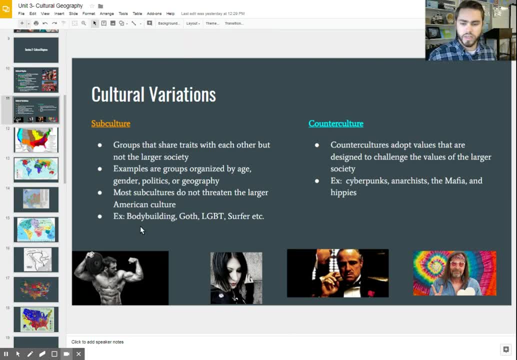 For example, you know bodybuilding. that is a subculture where they share that trait of you know constantly you know improving their bodies and trying to have the best you know shaped body possible. This is something that you know. while many Americans may do, they take it and really form. 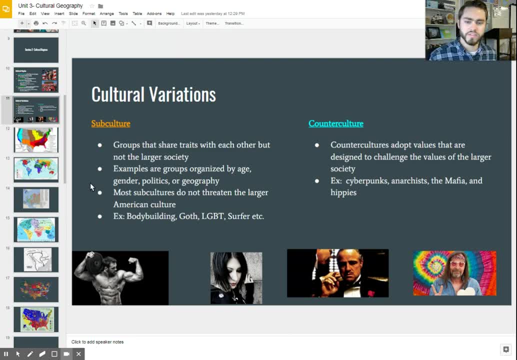 it as part of their true identity and culture, And so this would be a subculture that you know, while they are probably people in this bodybuilding culture are very similar to other Americans, in that respect they are a subgroup. Others you can see here goth LGBT surfer culture. 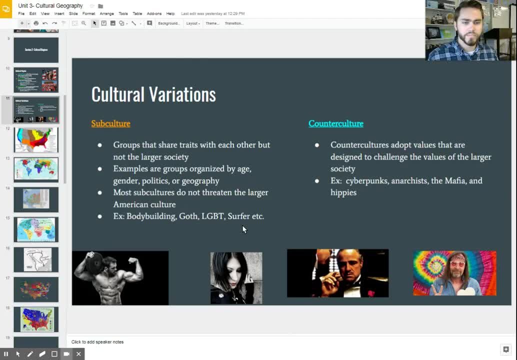 they all have different aspects of their culture that is both American but also, you know, different, And so that variation is what we call a subculture. They don't typically dislike other parts of American culture. The subcultures do. They're not going against American or other types of countries' culture. 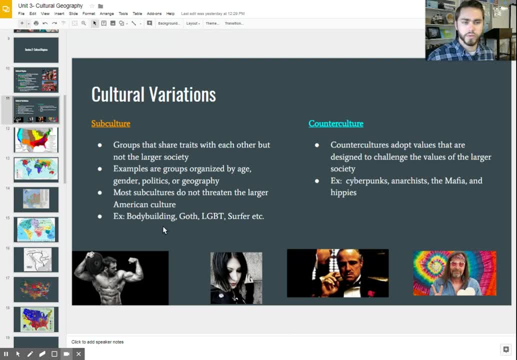 However, they do have a slight variance in one particular trait. The flip side of that is a counterculture. This is a culture that goes against the norm in society. So those norms that we talked about earlier in this unit, they're the ones that actively go against those values. 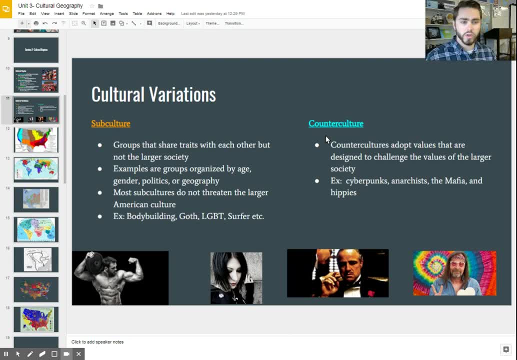 values, values, values And norms set by society as a whole, the large scale American community, And so countercultures, are ones that challenge those preconceptions, those norms in society. Probably a good example you probably know of are hippies. 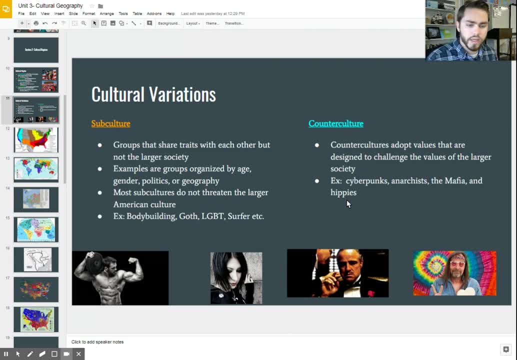 This is during the 60s and 70s movement, where they rallied against the government and many things, such as the war in Vietnam, And so they're going against traditional American cultures in that way, which makes them a counterculture, Same way in which a mafia member, you know, breaking, obviously, multiple laws would be an example of counterculture. 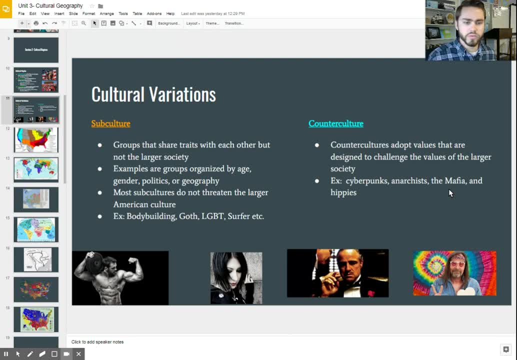 Ones that believe that the normal American values are wrong or necessarily they're going against them. Any type of group that does that would be considered a counterculture. Okay, So try to think of some others. you know groups that that might fall into that category. 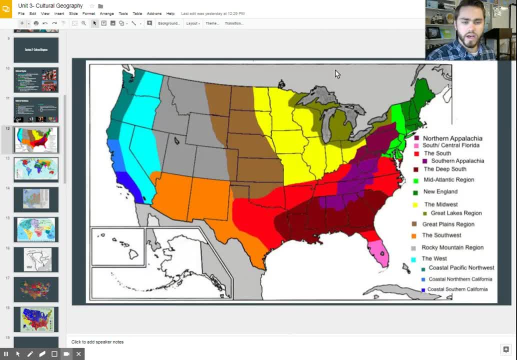 All right, Let's take a look at some of these groups. Let's take a look at some of the different ways in which we can map these subgroups or cultural traits. Here's a map Here. it shows where people are culturally similar, but also it tries to group people based on geography as well. 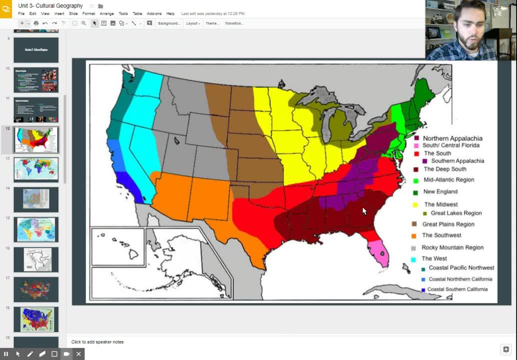 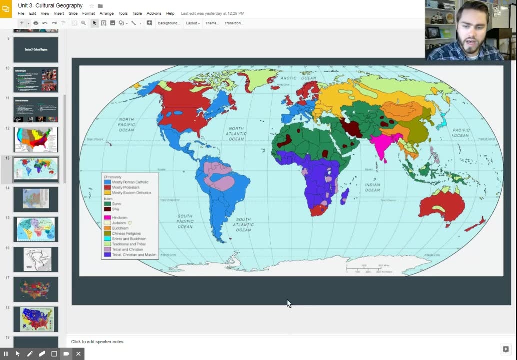 And we can see different groups here, such as the Deep South, where we are located here. But it even breaks down the South into different subregions to try to to narrow down where people are more similar to others. Another example here: This is a another thematic map that is showing particular religions and where they're predominantly located. 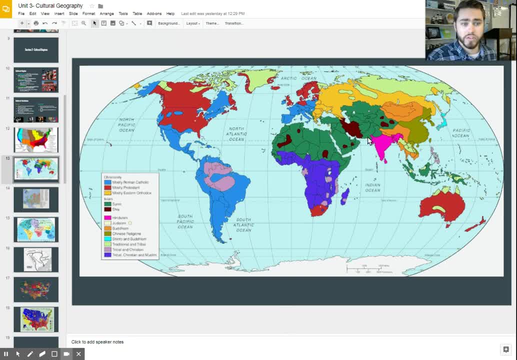 And so this is another way in which we can see data points mapped out across space, And in this particular data point we're looking at is religion, And so we can see where different cultural groups are the same, And so we can see what they have in common there. 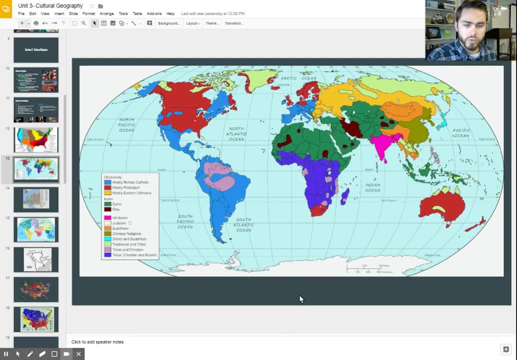 And we can understand the world a little bit better based on these different types of cultural traits. We know people that are, You know, Catholic here, also Catholic here and Catholic here, And so they share that trait in common, and we know more about how people are around the world. 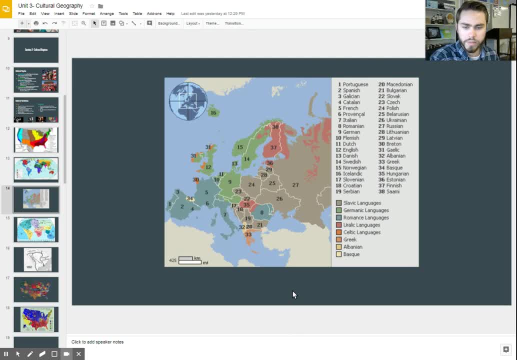 Here is another type. This is based on language, So where people share a common language family, these Romance languages, like you see Spanish, Italian or French mixed with. You also see Germanic languages. You can see English as a Germanic language as well as, obviously, German. 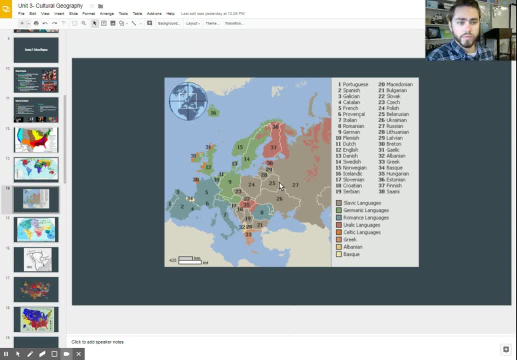 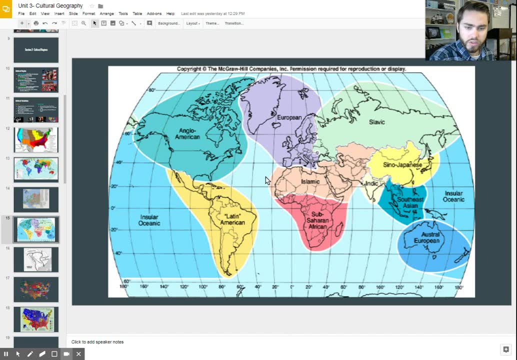 And some of these Others in northern Europe, And so you can see where, culturally, they share parts in common as well. Again, language: we're looking at not only language, but also, you know, different types of cultures here as well. 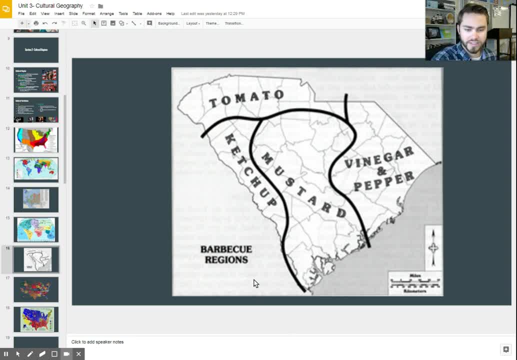 Here's an interesting one a little closer to home. This is, as you can see, a region based on barbecue, And this is where people in different areas of the state prefer their sauce to be. You know, derived from? or do you want a mustard based sauce? here in the Midlands, like is most common vinegar pepper, where I used to live in in Horry County, is the only kind that you'll find there along the coast. 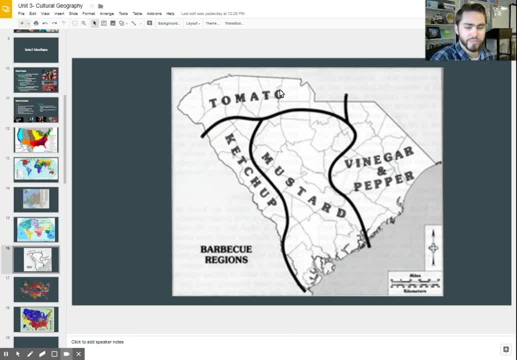 And I believe that one's the best- where in the upstate you see more tomato based sauces, And so you can tell more about people's culture just on particular cultural traits such as that. Here's one of my favorite ones. Take a minute and see if you can figure out what this is. 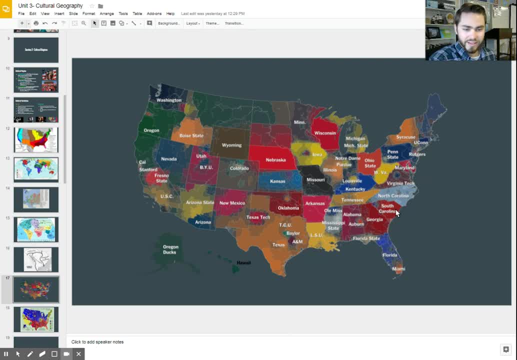 All right. this is, as you may or may not have guessed, based on college football team preference And if you, if you look closely, it's very based on not just the state as a whole, but different regions of the states and what their favorite football teams are. 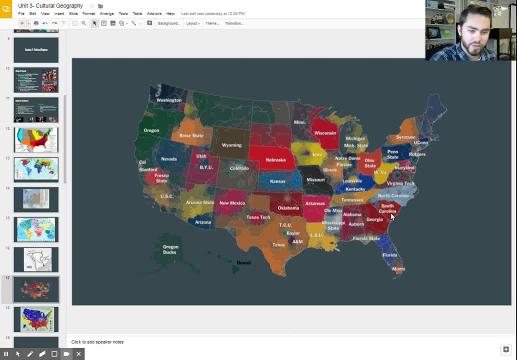 And so you can see in South Carolina, predominantly in this half of the state it's going to be South Carolina and in the northern half it's Clemson, And you can see that for Different teams around there as well, And so we know more about different particular cultures based on that trait.